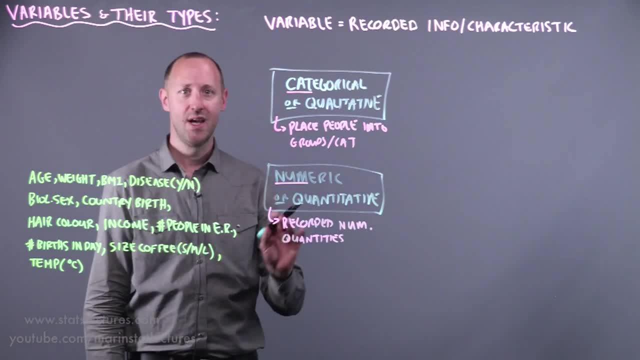 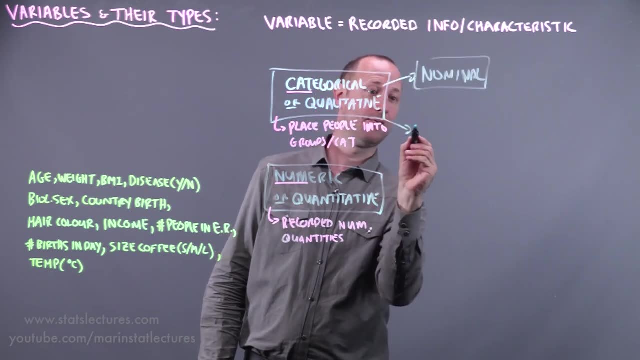 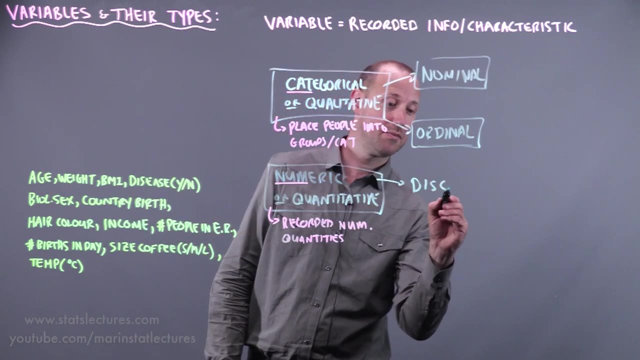 about how these can be further broken down. So categorical variables can be further broken down into what we call nominal or ordinal, And numeric variables can be further broken down into discrete. so I'm just going to summarize that D-I-S-C or continuous. Again, I'll just 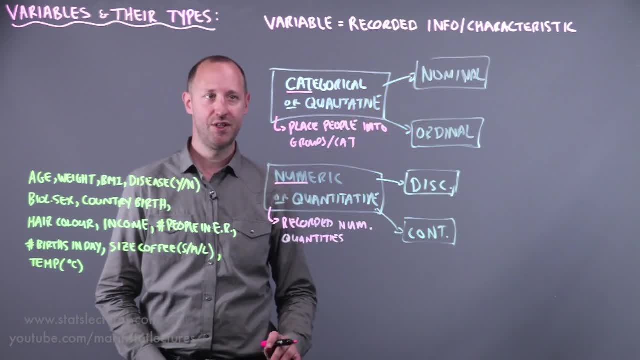 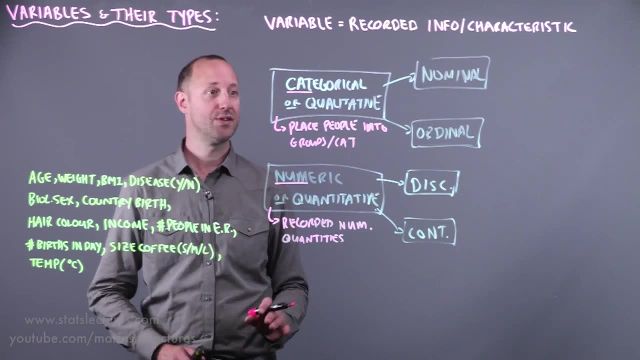 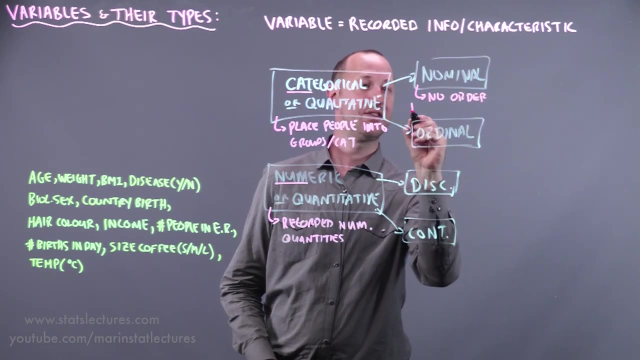 abbreviate that C-O-N-T. Okay, so let's talk about each of these Categorical variables, things like biological sex right- male or female- country of birth, these sorts of things. Nominal means that there is no ordering based on magnitude. 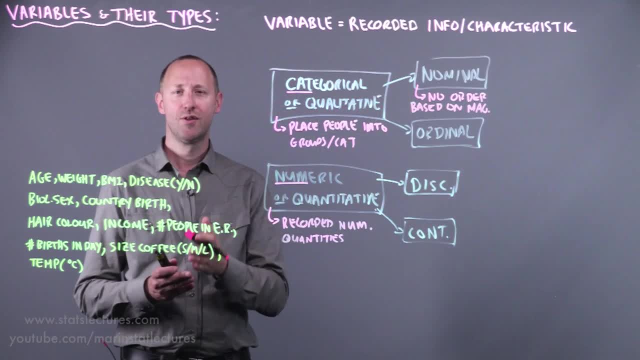 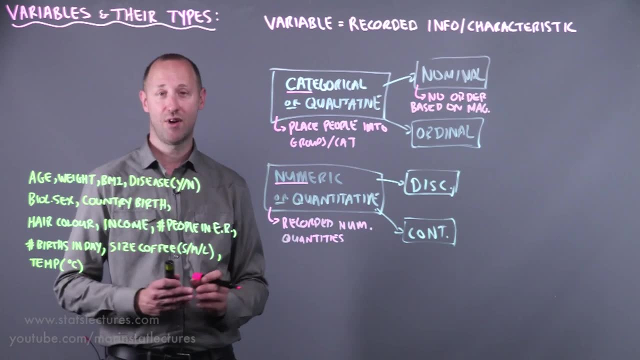 or size. So country of birth? there's no, you can order them alphabetically, but there's no smallest to largest ordering Where, if you think of something like the size of coffee, that someone orders, right, that's categorical: small, medium or large, but there is an ordering. 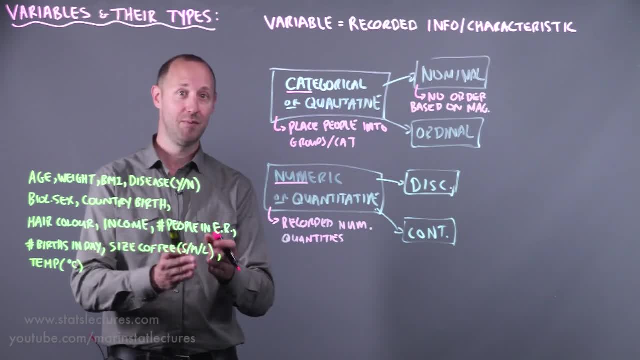 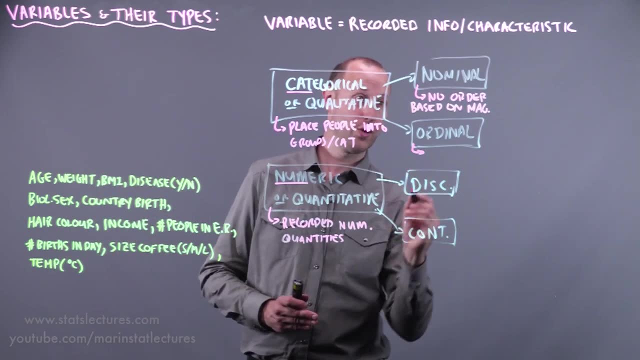 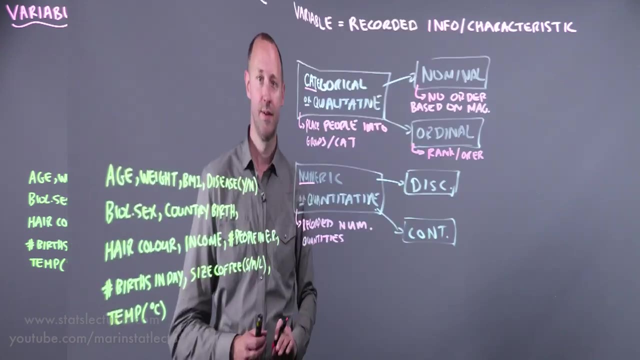 based on the size or magnitude. Small is smaller than medium, Medium is smaller than large. So there is an ordering or a ranking to these categories. So that's what we call ordinal. There is a rank or an ordering- Discrete and continuous. it's a bit more of a gray area between these two and they're 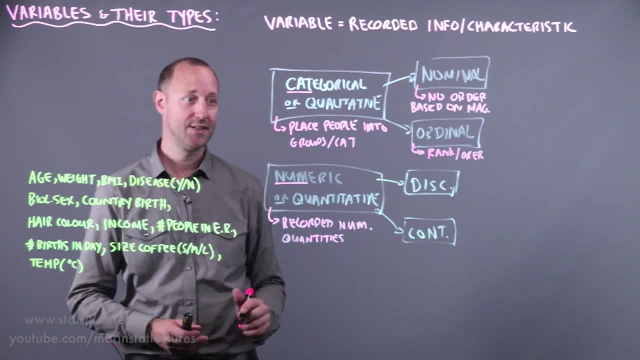 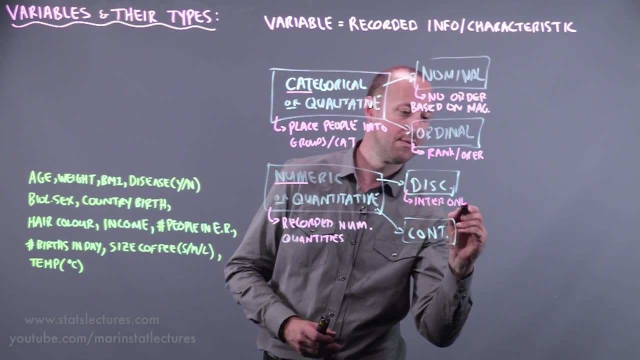 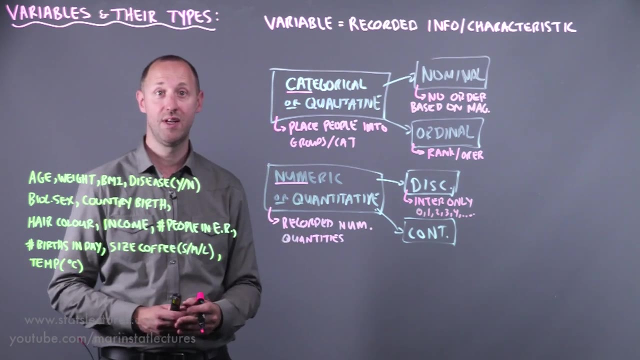 often treated the same or very similarly in analysis. but discrete variables tend to take on integer only, So things like take on a value of zero, one, two, three, four. In theory they can go all the way up to infinity, but integer only, So things like the number of 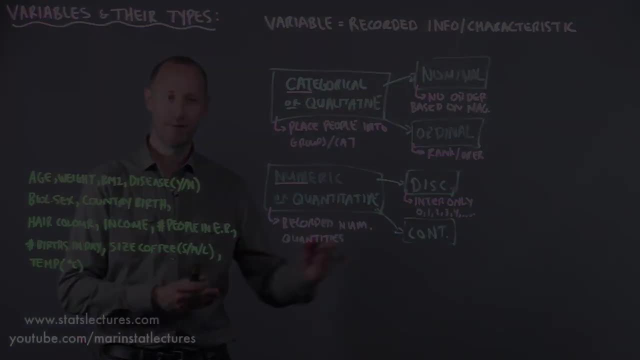 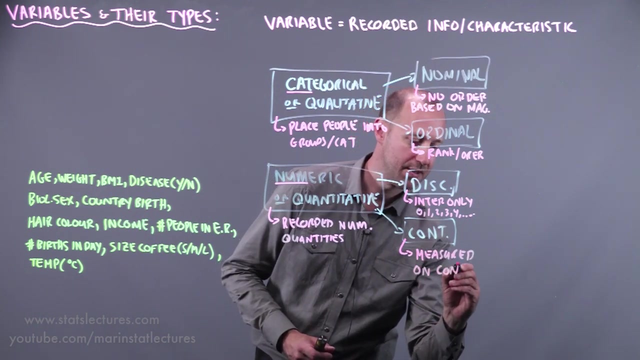 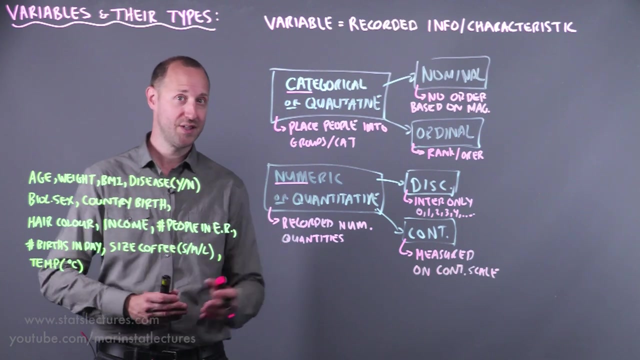 people who are in an emergency room. There's zero or one or two Continuous variables. these are measured on a continuous scale. So when we record someone's weight, say, We often report weights to the nearest pound or nearest kilogram. but they're. 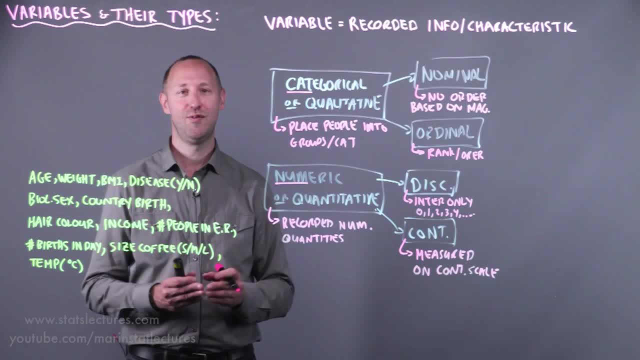 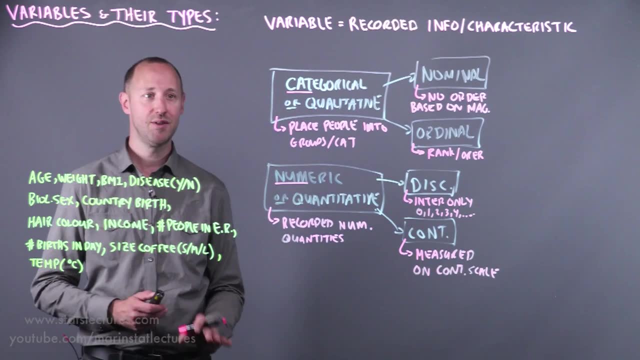 actually measured on a continuous scale. right, Your weight can be 57.258 kilograms, for example. So what we're going to do now is go through and take this list of variables and decide whether they're categorical or numeric. So what we're going to do now is go through and take this list of variables and decide. 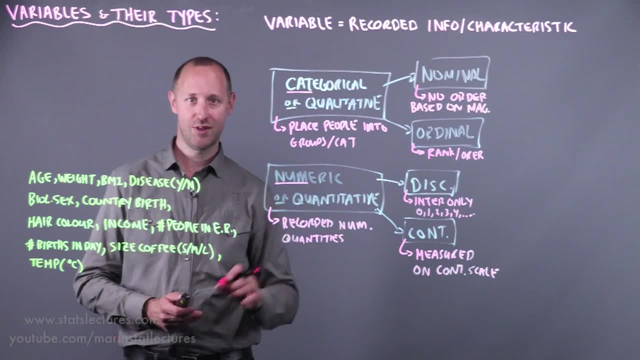 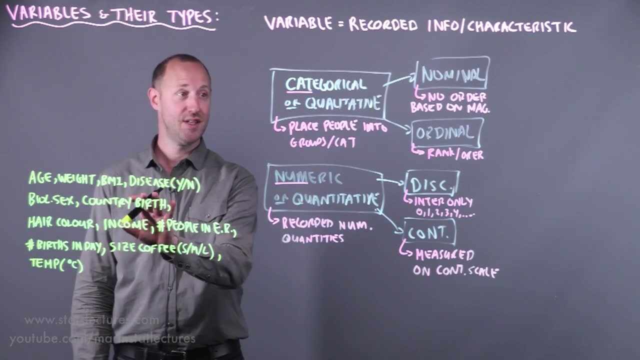 whether they're categorical or numeric, And you might want to take a moment to pause the video and try and do this yourself before looking at me. do this, Okay. so let's go through and place each of these variables into which type we think they. 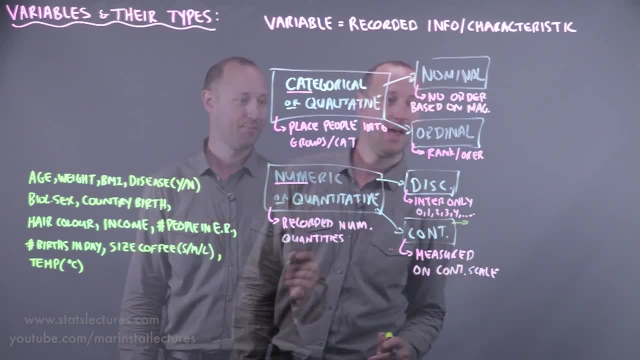 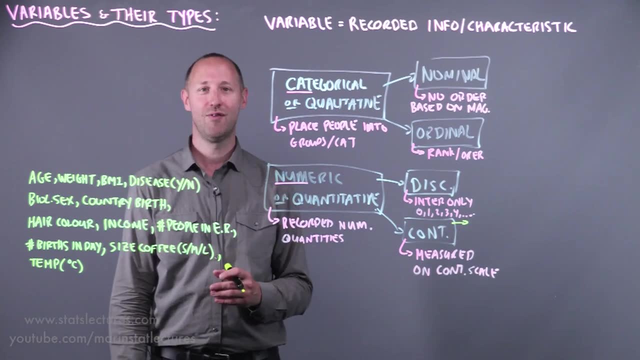 are. So age right is a recorded quantity and it's continuous. Again, while we report our age to the nearest whole number, no one ever says that they're 35.738 years old, but it actually is measured on a continuous scale. So again, we look at the number of people who are in an emergency room and then we go to the next one. So the number of people who are in an emergency room and then we look at the number of people who are in an emergency room. 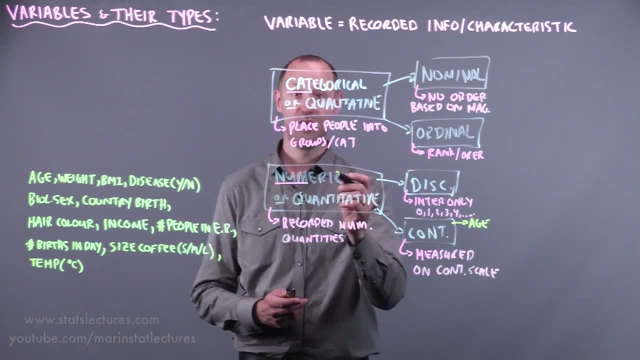 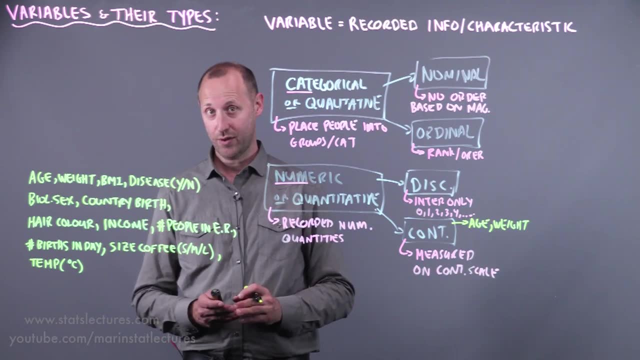 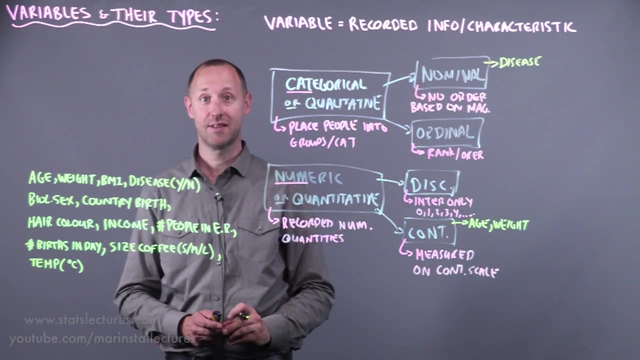 continuous scale. Now thinking about weight again, that's a numeric measurement and it's on a continuous scale. What else Disease recorded as yes or no? that's categorical right. we're placing someone into categories and there's no ordering or rank to these Biological sex right, again, recorded as: 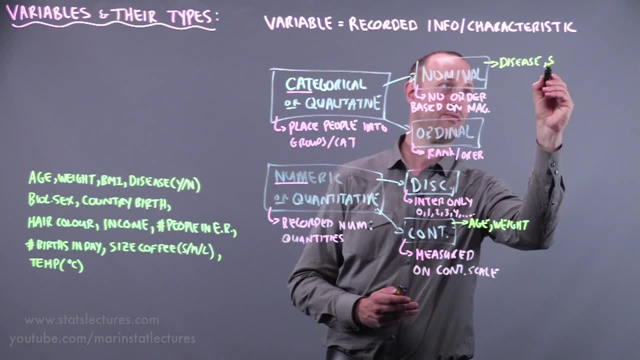 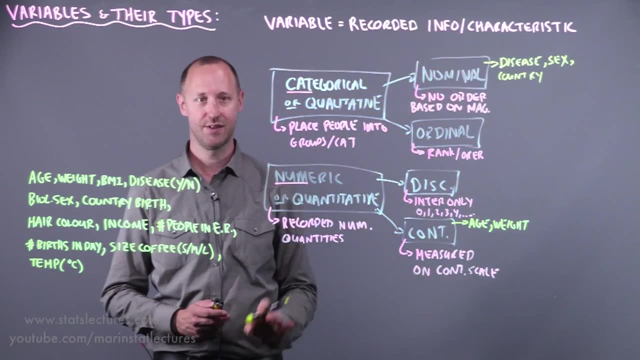 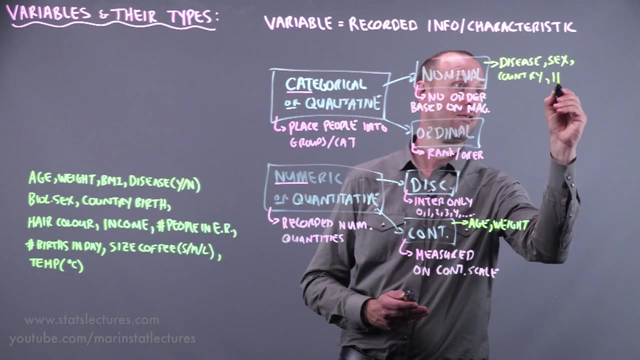 male or female. that's a nominal, categorical, variable. Country of birth. I'll just shorten it right country here, just for the sake of space. Hair color: again right, it's categorical, it's nominal, right. no natural ordering to. 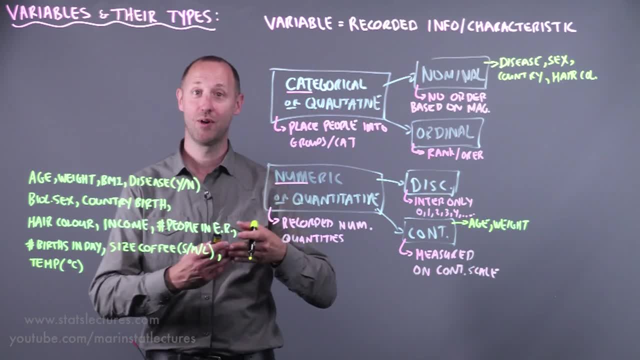 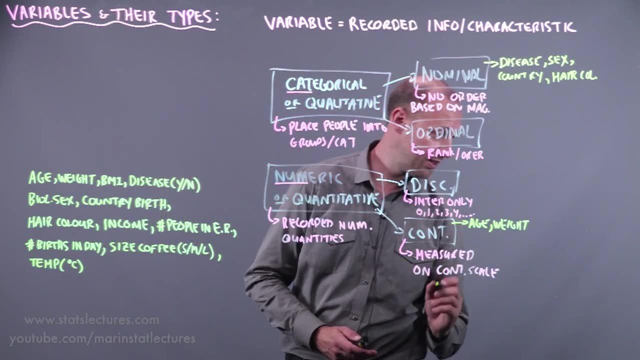 these. Again, you can order them alphabetically, but we're talking about a ranking based on size or magnitude. Income- again, that's a continuous variable. What else you have? The number of people in the emergency room right, or, again, number of people maybe. 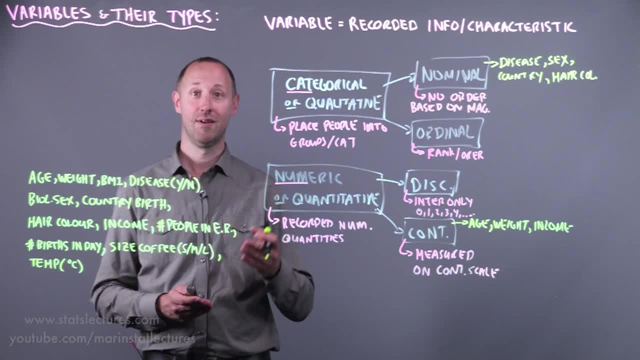 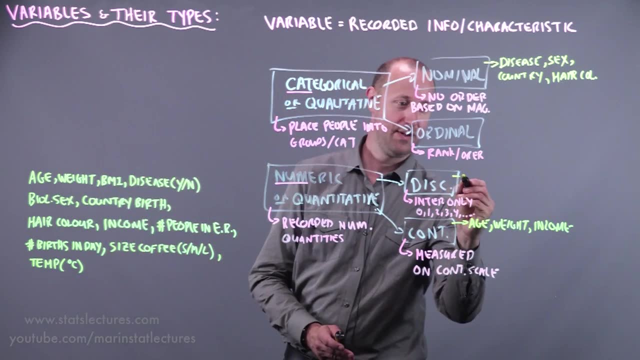 a number of people at a moment in time, or a number of people that show up in a day right, this is a quantity or a numeric variable and it's discrete. It's gonna be zero or one or two or three in theory, and go up to infinity. The number of live. 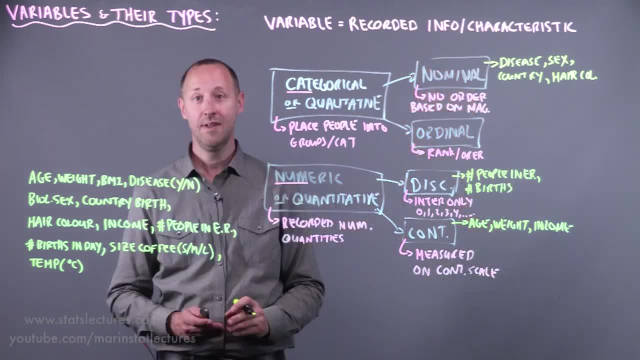 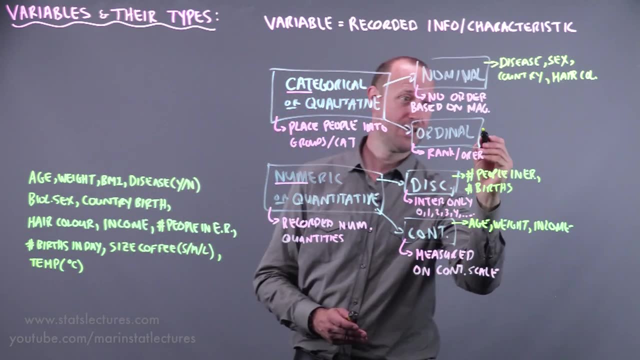 births in a day in a hospital- again, that's discrete. The size of coffee that you buy, small, medium or large, right, that's a categorical variable and there is an ordering or ranking to these. And finally, temperature, recorded in degrees. 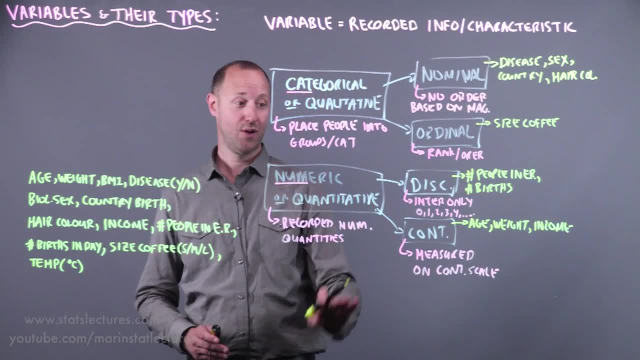 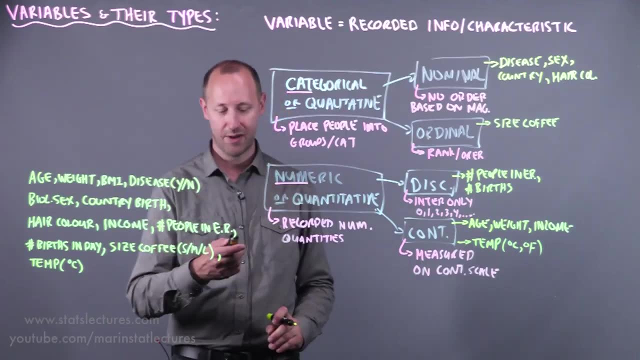 Celsius or degrees Fahrenheit doesn't matter. right, that's a numeric quantity and, again, measured on a continuous scale: Degrees Celsius, or you could put it as degrees Fahrenheit, doesn't really matter. Now a few important things to note before we continue on. The first is that categorical variables. 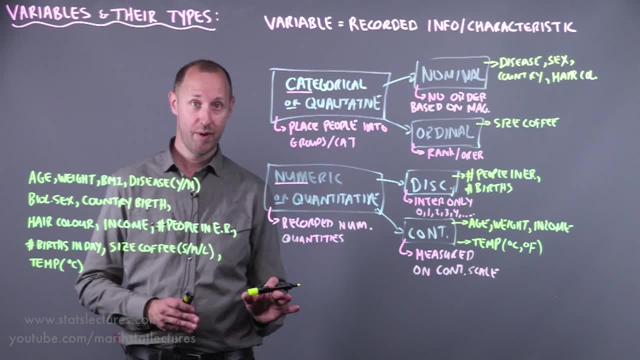 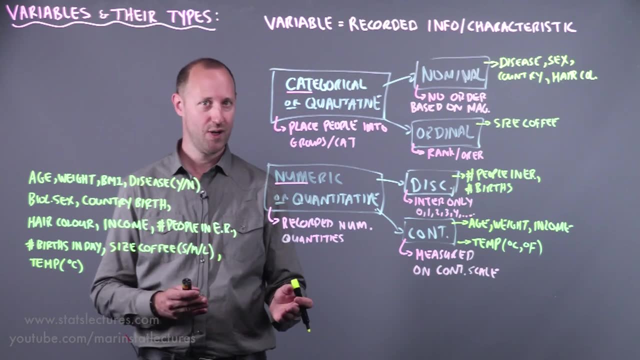 sometimes are recorded using numbers, but that doesn't make them numeric. So quite often with things like does someone have a disease, yes or no, they often get recorded with zeros and ones, One, often indicating yes they do, zero they don't, Or biological. 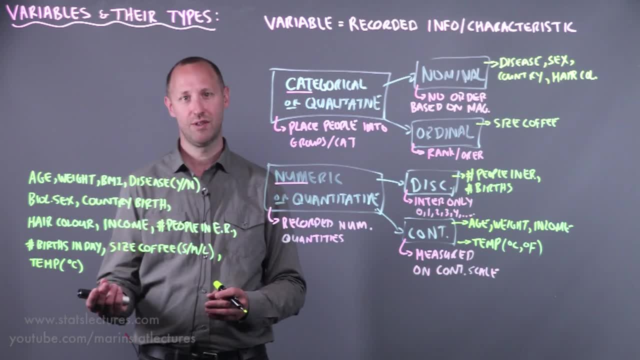 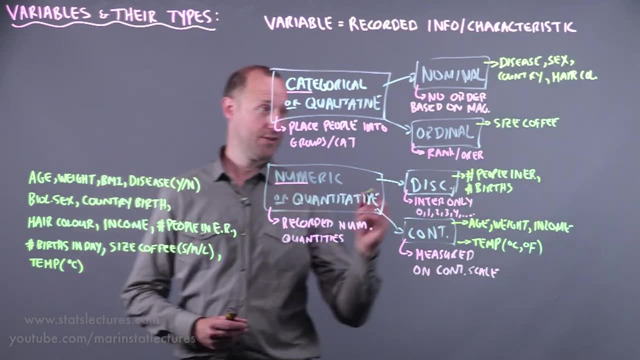 sex right, male and female. We might record males with zero, females with one, but again, these are not numeric variables, we're just using numbers to record them. Another good example is the Likert scale. So again, this is where we 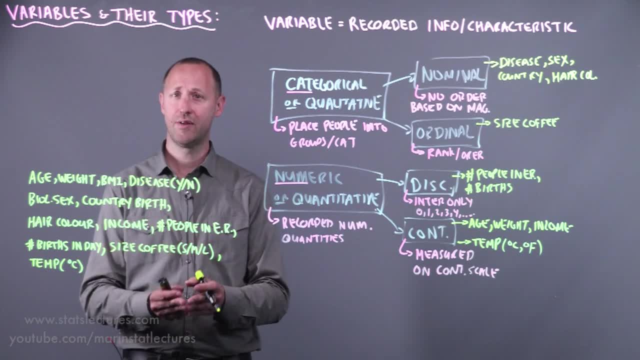 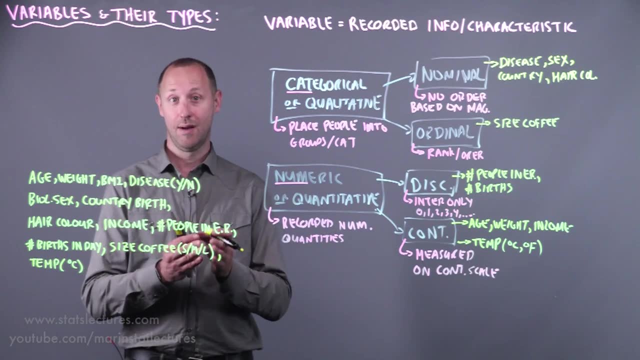 ask people: do you strongly disagree, disagree, neutral agree, strongly agree? And we often ask them to rank it using one, two, three, four or five. So there we're, using numbers to indicate categories, right levels of agreement or 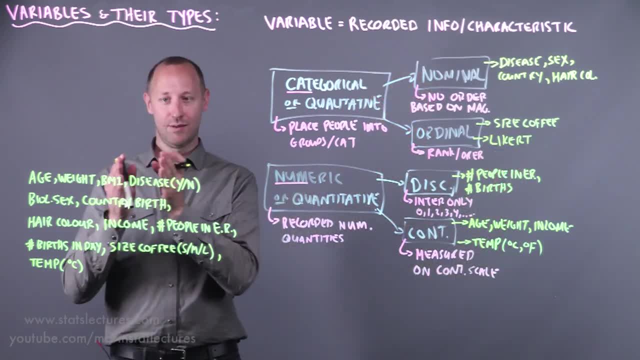 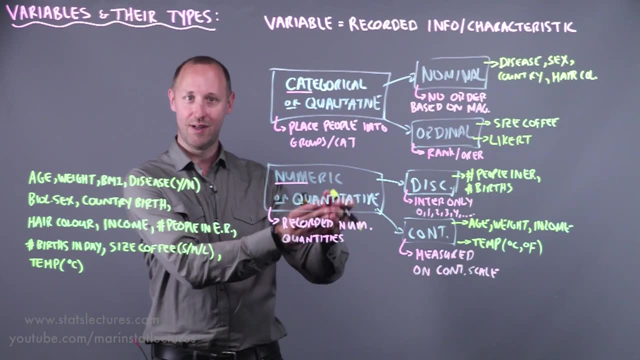 disagreement. And so there we're looking at an ordinal variable- Strongly disagree- and then a little bit higher than that is disagreeing and a bit higher is neutral and higher is agree and higher is strongly agree. right, So there's a ranking or ordering to those but the 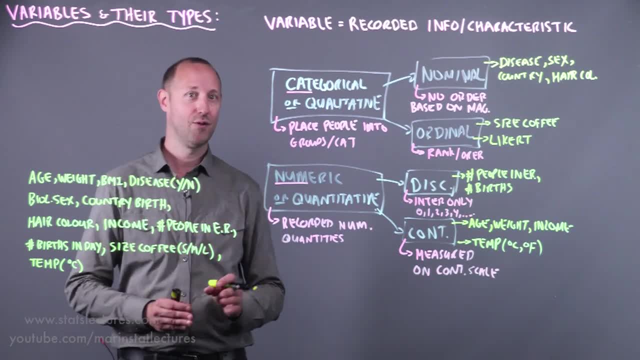 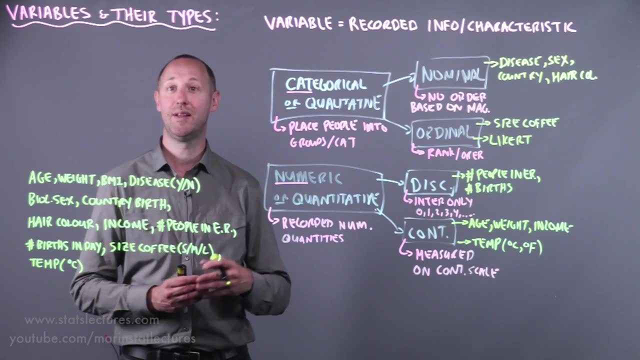 numbers don't actually mean anything other than being labels for these categories. Another example we can look at is suppose we all decide to go and do a 10 kilometer race together, So we can record how long did it take us to finish the race right And this: 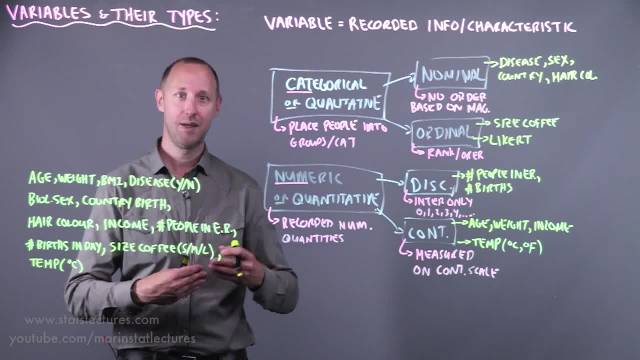 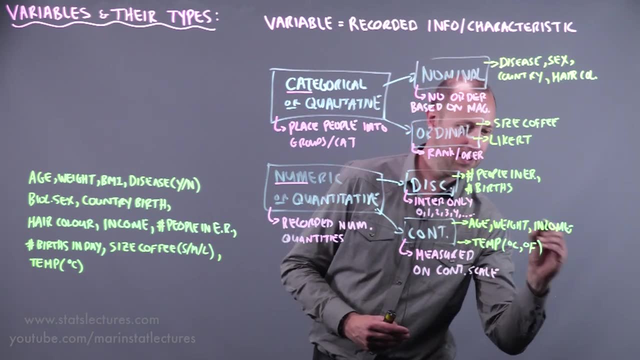 variable is a numeric measurement, right, We're recording how many minutes and seconds did it take us to run 10 kilometers? So that's a continuous variable. So I'm going to add that in here. the race time: right Again: how many? 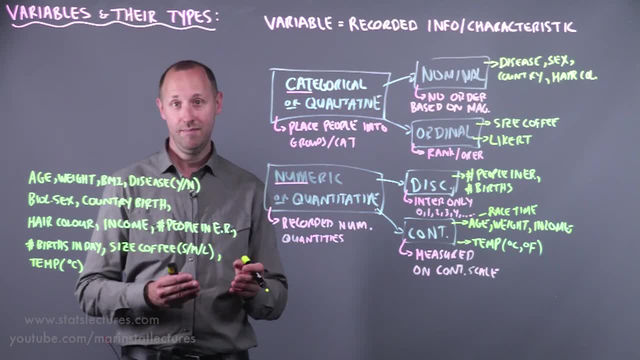 minutes and seconds. did it take you to finish the race? If we make it competitive and look at who finished in first, who finished in second, who finished in third and so on, right Now we're looking at categories, right We're. 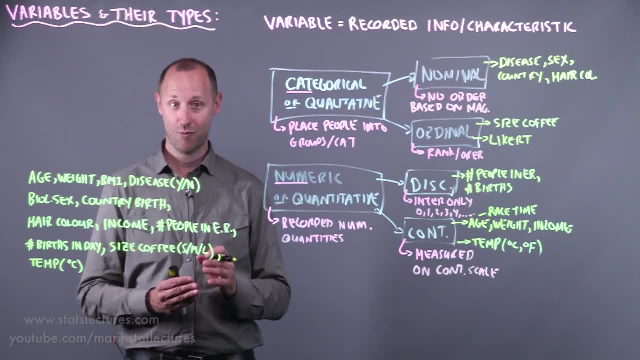 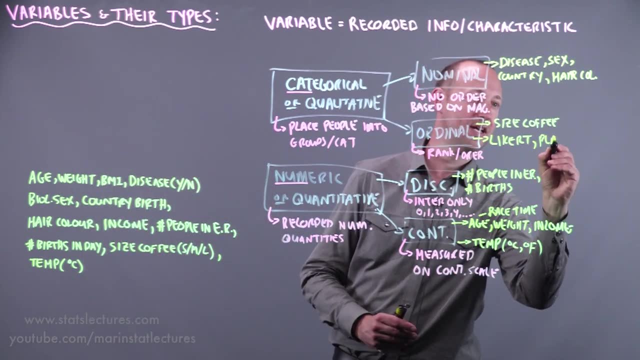 looking at the place that people finished, and there is a ranking to these. First place was the fastest, second was the next fastest, third was the next fastest. So here the place that someone finishes in a race is a categorical variable and it's ordinal right. There's a ranking to them, And so 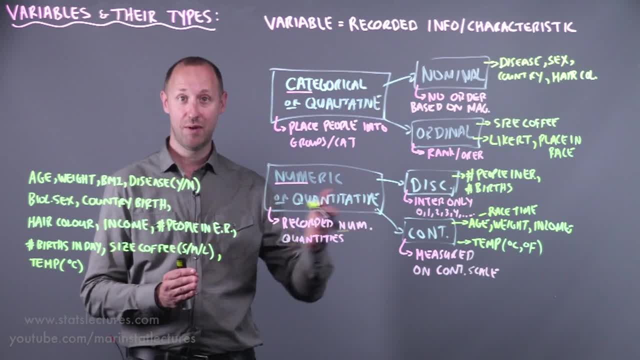 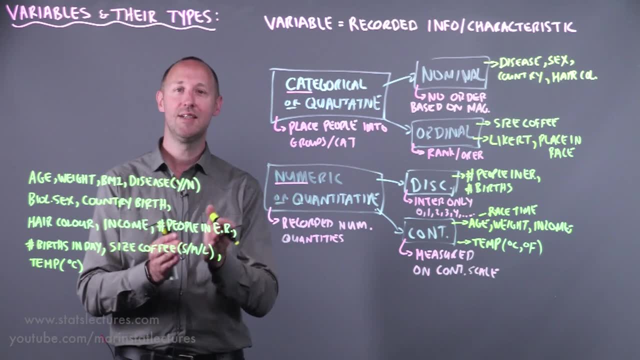 again, a feature of ordinal variables is, while the categories can be ordered or ranked, the spacing between them is not necessarily equal right. The distance between first and second place isn't necessarily the same as the distance between second and third, or the distance between third and fourth, and so on. 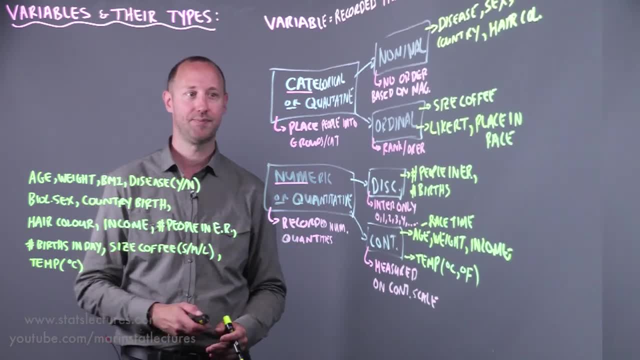 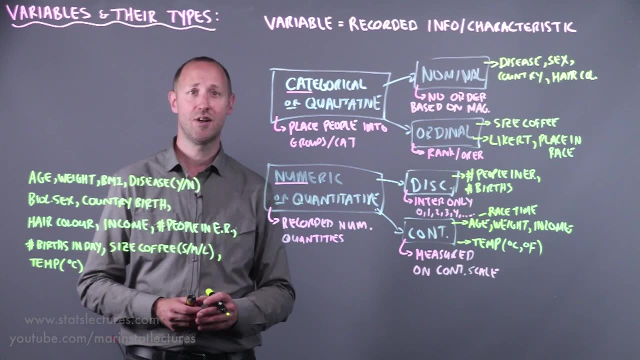 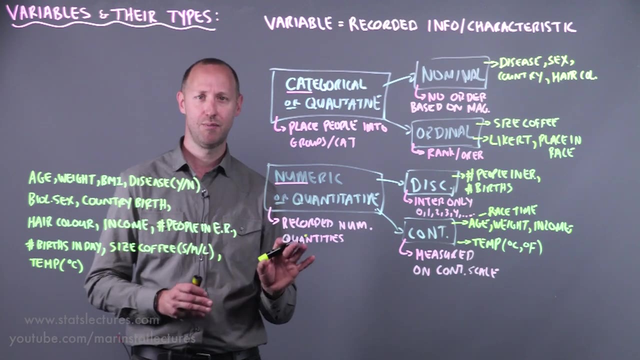 Right, so these are rank variables or ordinal variables. So, as we mentioned before, the sorts of plots that we make the summaries of the method of analysis depends largely on are we working with categorical variables, numeric, or what combination of categorical and numeric? Okay, so it's important to to make this. 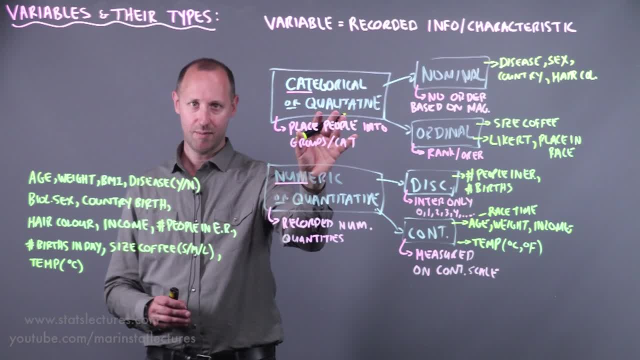 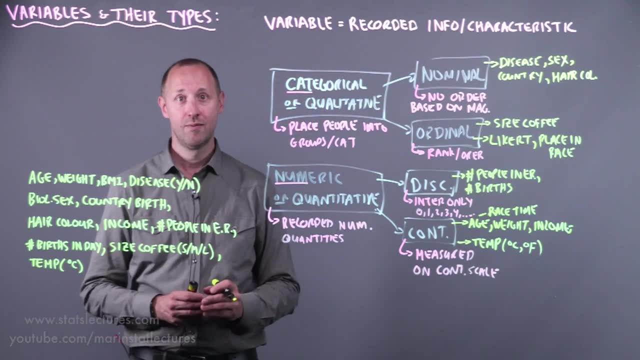 distinction. now A quick mention: Categorical variables often get summarized using proportions or percentages. So if we're looking at, let's just say, biological sex, we often get categorical variables summarized using conditions or percentages. So if we're looking at, let's just say, biological sex, we 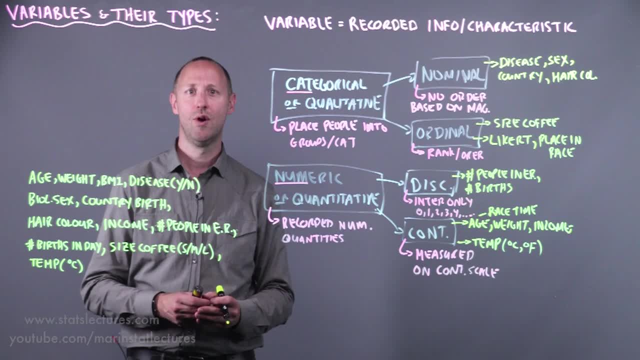 often summarize that by looking at how many males and how many females or what percentage of males and percentage of females were there Numeric variables. if we're looking at, say, something like age, we often summarize that using the mean or average age or the median age. Okay, so in following videos we start to talk. 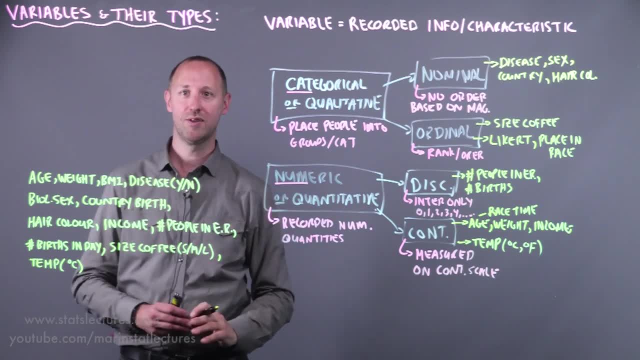 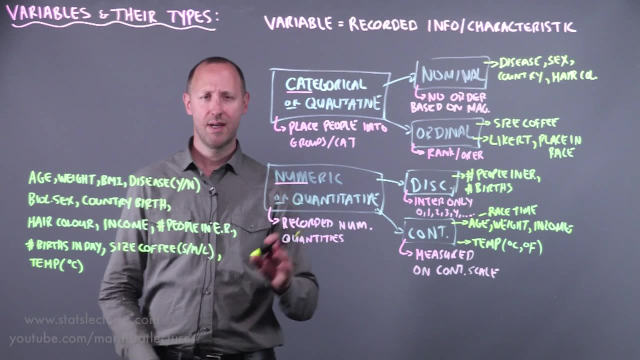 about appropriate summaries for categorical or numeric variables, appropriate methods of analysis and so on. Now one more important note, and this really becomes a little bit more important further down the line, but we're going to mention it now mostly for the the sake of completeness. Discrete or 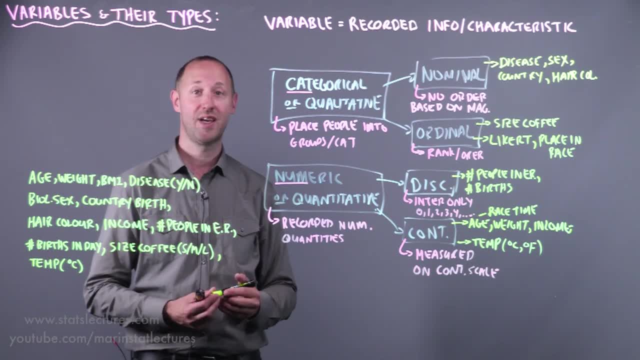 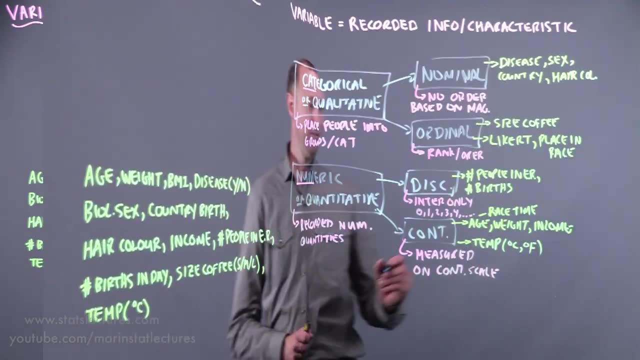 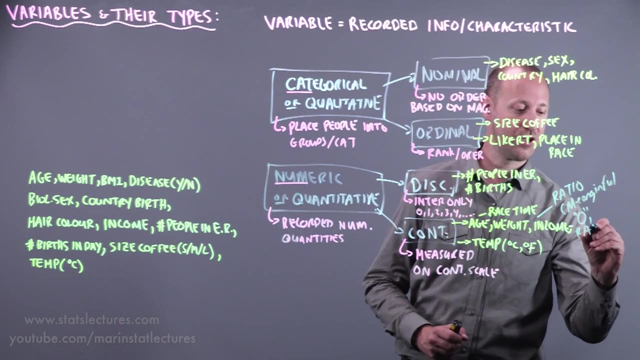 continuous variables can be further subdivided into scales of measurement, looking at the ratio scale or the interval scale. Okay, so let's quickly mention what those are. So the ratio scale has a meaningful zero or a meaningful ratio, And what that means is, if we look at these variables here- age, 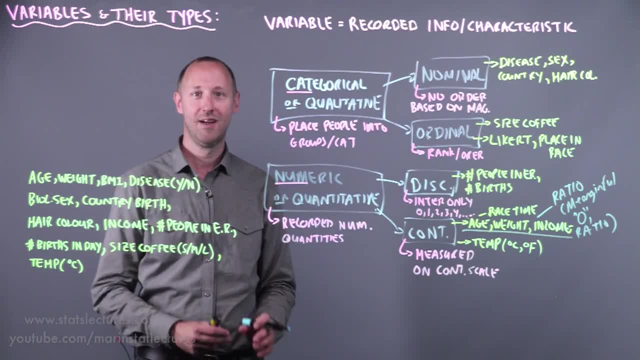 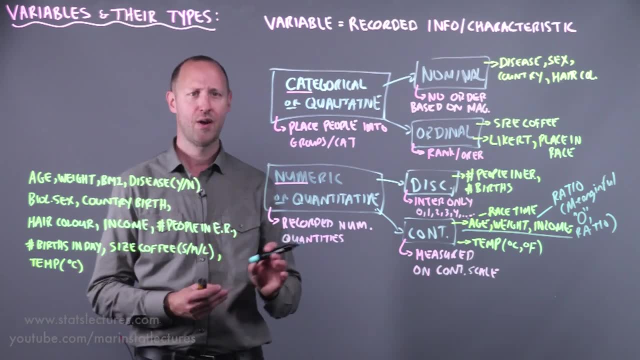 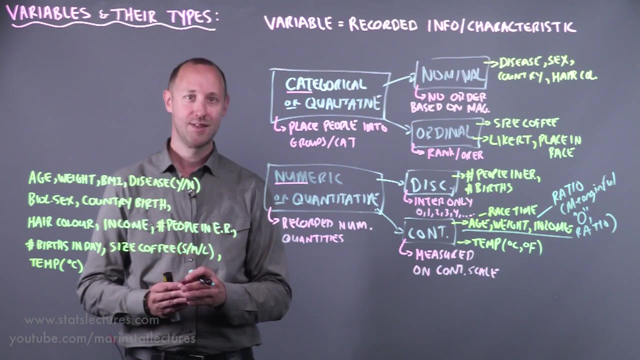 weight, income. they're measured on a ratio scale, Meaning an age of zero. is that zero means something right? There is no age Or a weight of zero. there is no weight- Another way to think of it- a ratio is meaningful. Someone who's 20 years old is twice as old as a 10 year old Someone. 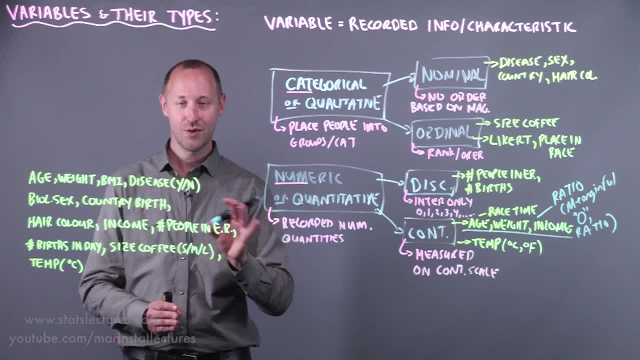 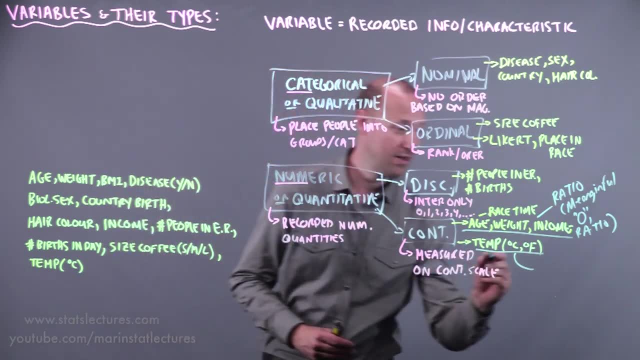 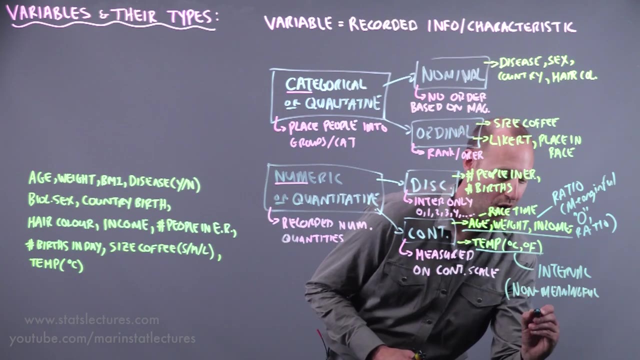 who's 30 is twice as old as a 15 year old, So that ratio makes sense. Things like temperature can measured on degrees Celsius, or degrees Fahrenheit are measured on what we call an interval scale. This has a non-meaningful or an arbitrary zero, And again, what we mean by that is. 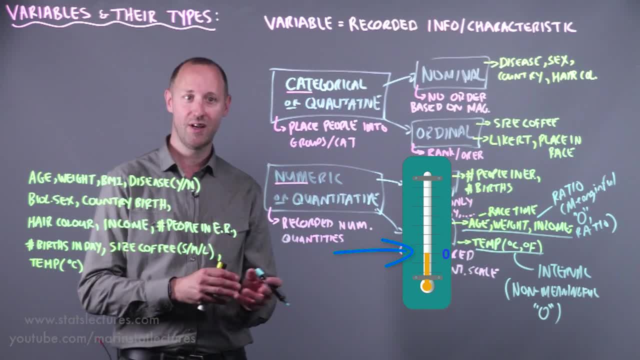 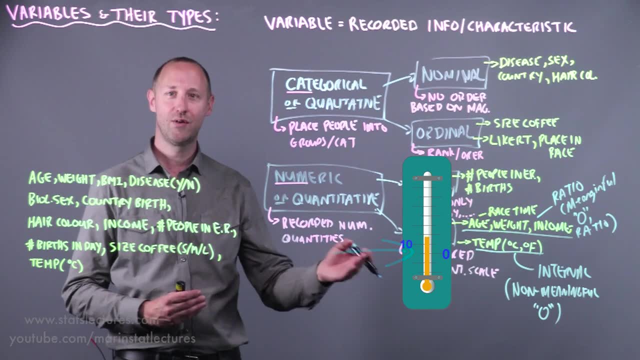 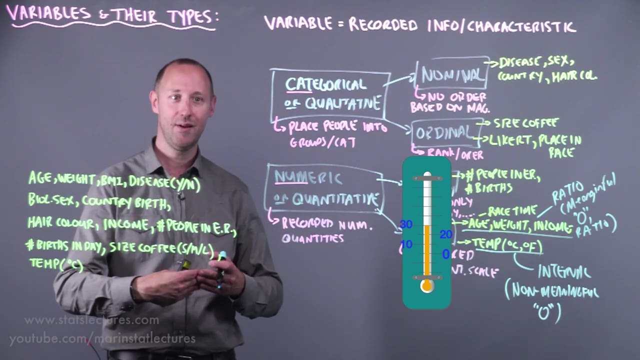 a temperature of zero degrees Celsius or zero degrees Fahrenheit doesn't mean there's an absence of temperature Or they do not have a meaningful ratio. 20 degrees is not twice as hot as 10 degrees. 30 degrees is not twice as hot as 15 degrees. This is a scale, but the zero is not an absence. The 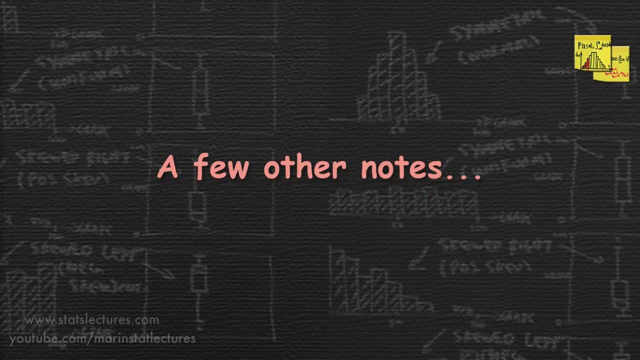 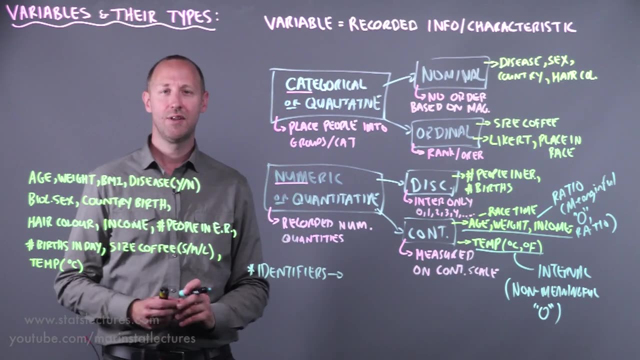 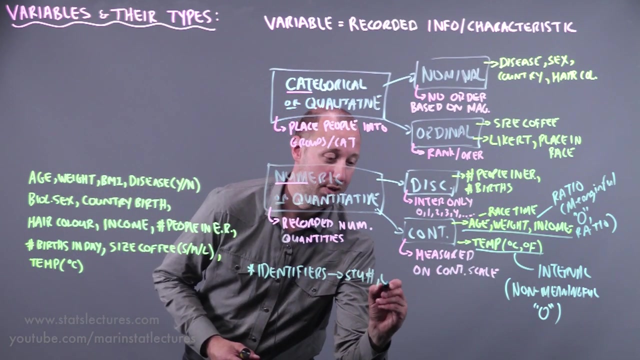 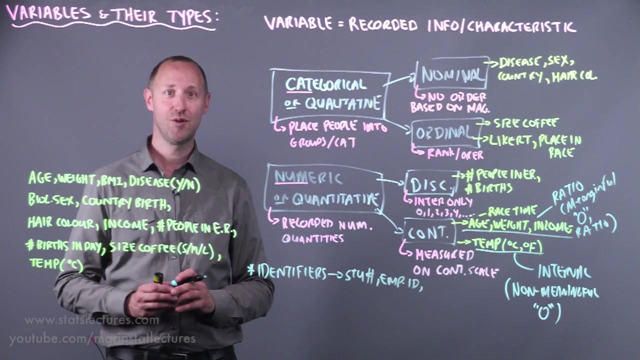 ratio is not meaningful. Now, just a few other important notes for us to talk about before we wrap this up. The first is identifiers. So often there's identifiers that are used- Things like your student number or an employee ID, Things like these. These are used to identify an individual, but they're not. 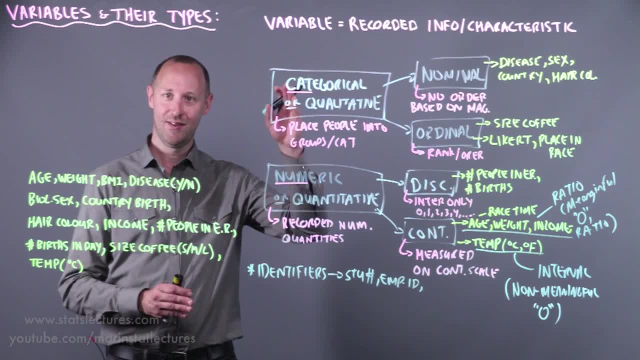 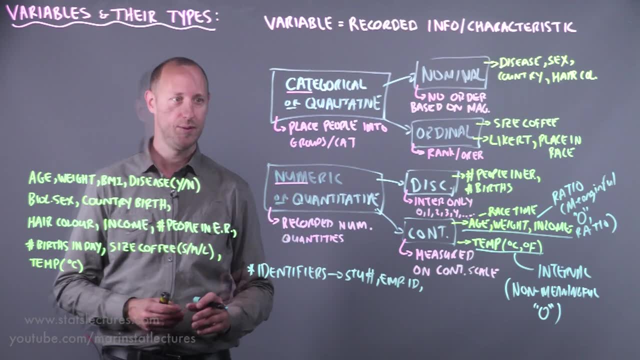 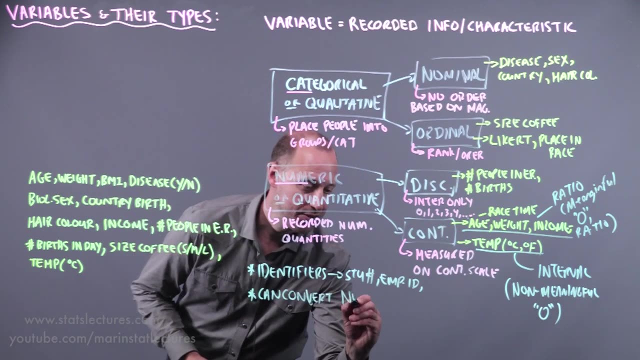 variables. They sometimes fit in this conversation in that they're often one of the columns in your data set, but they really used to identify an individual. They're not a true variable. Another important note is that you can always convert numeric variables into categorical variables. Okay, so for. 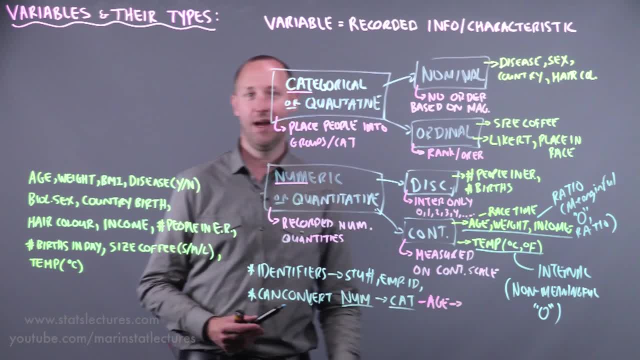 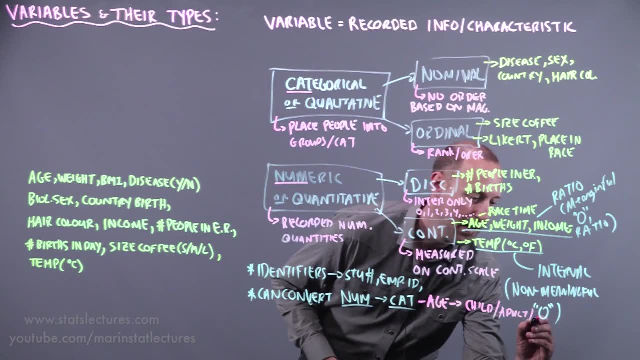 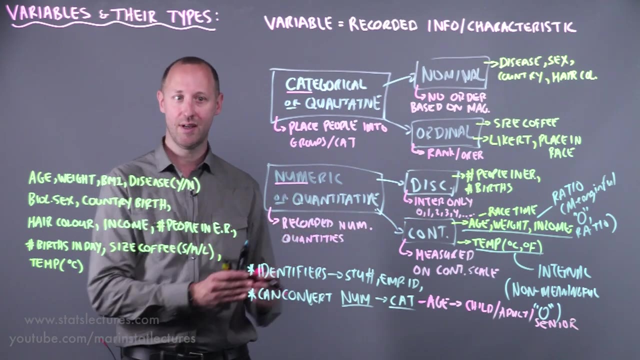 example, we can take something like age, And rather than using numeric age, we can convert that or break it down into, say child, adult and say senior, Or we might just break it into age categories of 0 to 10,, 10 to 20,, 20 to 30, and so on. And then, I guess, one final note to mention. 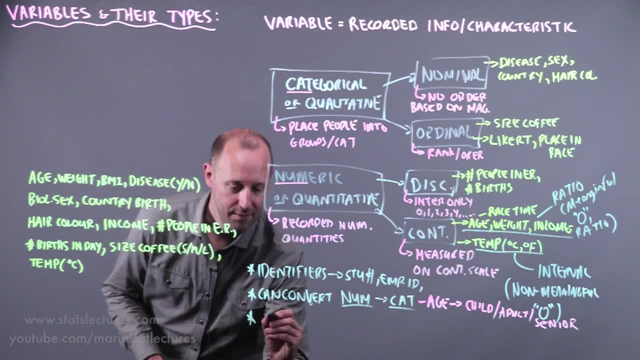 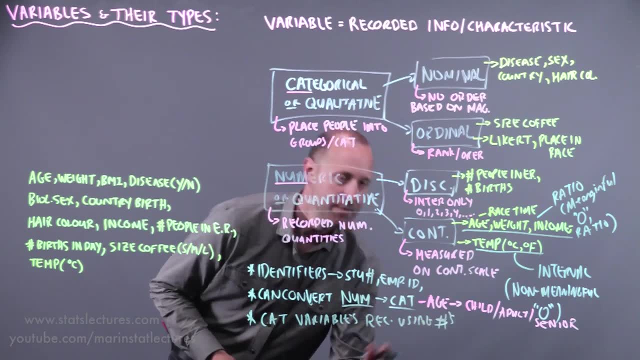 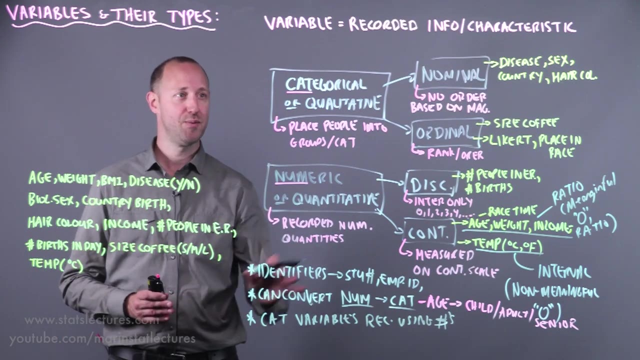 that we've already said, but I'm going to write it down here, is that sometimes categorical variables are recorded using numbers. This doesn't mean that they're numeric variables, but we often use numbers as placeholders for the categories. So in the following videos we start to explore.